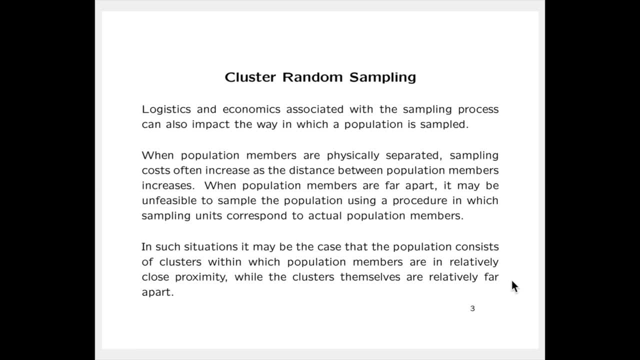 the distance between population members increases When population members are far apart. it may be unfeasible to sample the population using a procedure in which sampling units correspond to actual population members. In such situations, it may be the case that the population consists of clusters within which population members are in relatively close 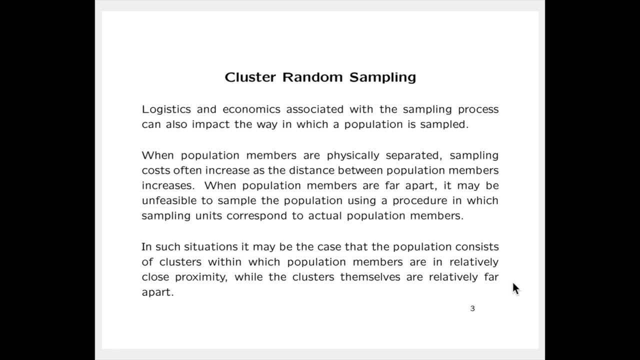 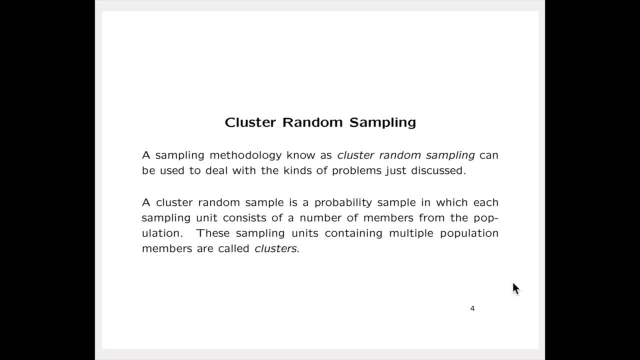 proximity clusters themselves are relatively far apart. A sampling methodology known as cluster random sampling can be used to deal with the kinds of problems just discussed. A cluster random sample is a probability sample in which each sampling unit consists of a number of members of the 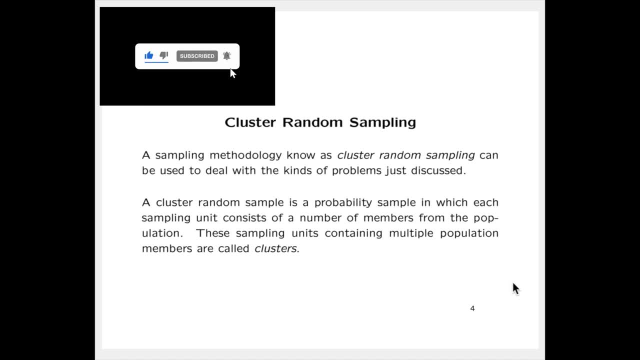 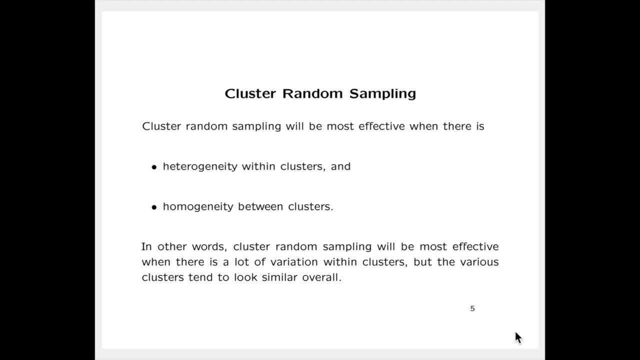 population. These sampling units containing multiple population members are called clusters. Now, cluster random sampling will be most effective when there is heterogeneity within clusters and homogeneity between clusters. In other words, cluster random sampling will be most effective when there is a lot of variation within clusters, but the various clusters tend 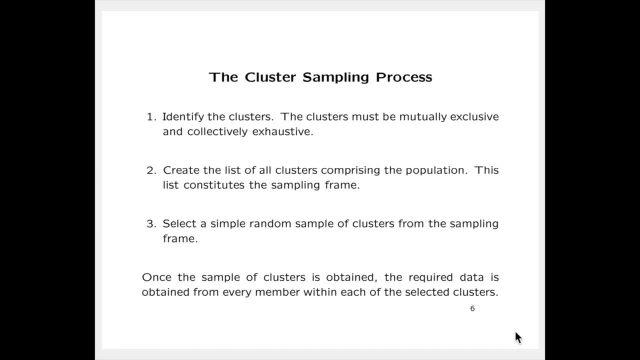 to look similar overall. Now here's the cluster sampling process. First, we have to identify the clusters. The clusters must be mutually exclusive and collectible. Number two: we need to create the list of all clusters comprising the population. This list, 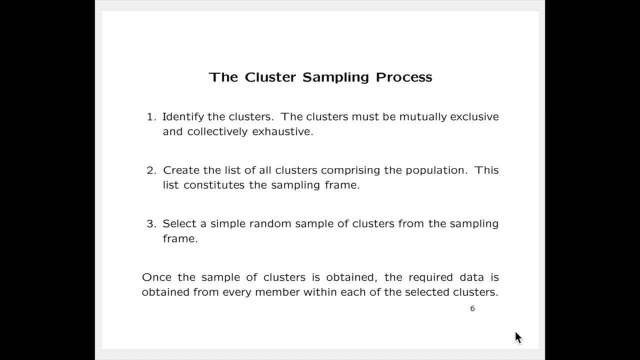 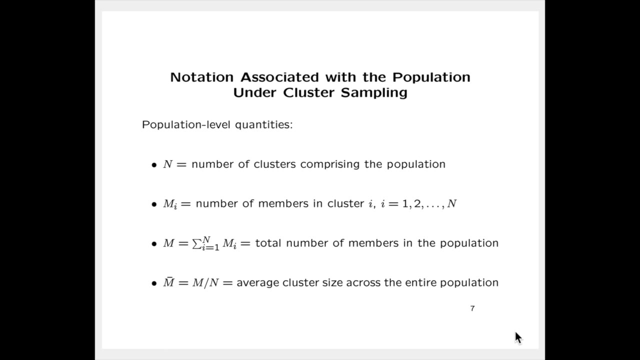 constitutes the sampling frame, And then three select a simple random sample of clusters from the sampling frame. Once the sample of clusters is obtained, the required data is obtained from every member within each of the selected clusters. Now here is some notation associated with cluster. 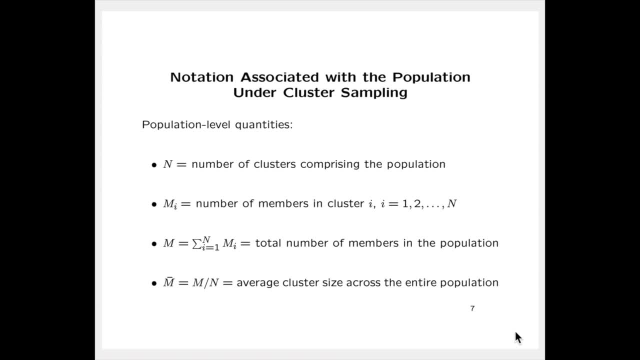 random sampling and these are population level quantities. The number of clusters comprising the population For each i going from 1 to n. m sub i, cap m sub i is the number of members within cluster i. The sum of the m sub i's cap m without a subscript. 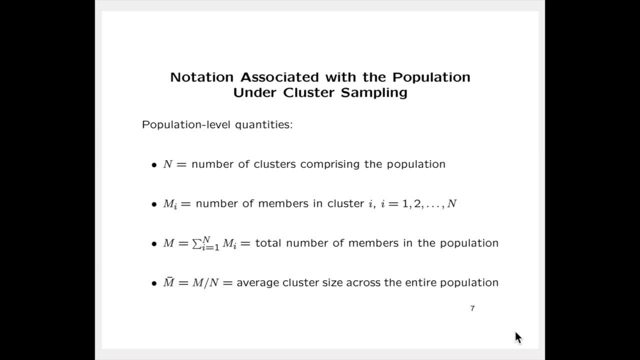 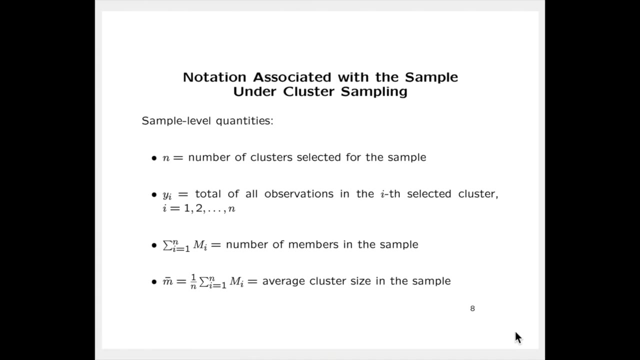 is the total number of members in the population. And then if we divide cap m by cap n, we're going to denote that ratio by cap m bar, and that is the average cluster size across the entire population. Then we have sample level quantities. Lowercase n is the number. 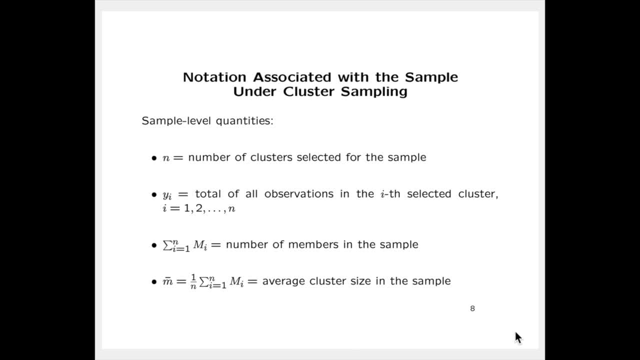 of clusters selected for the sample And then for each of the selected clusters. i going from 1 to little n y sub i is the total of all the observations in the ith selected cluster. In other words, it's the total of the observed response for all of the members in the ith. 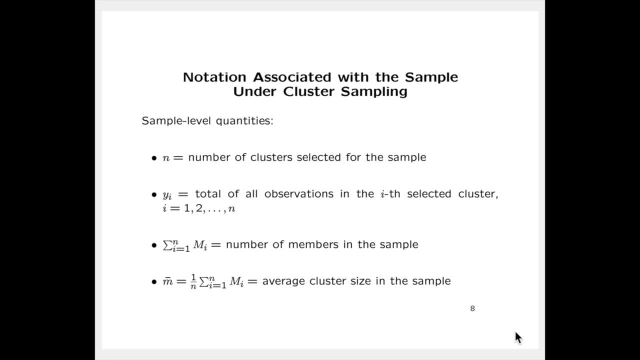 selected cluster, Then it shows us the number of twice the total down to m in the sample. and if we divide that by little n, by little m, which is the same as a cluster size in the sample. Now let's look at inferences for a population mean using cluster random sampling. 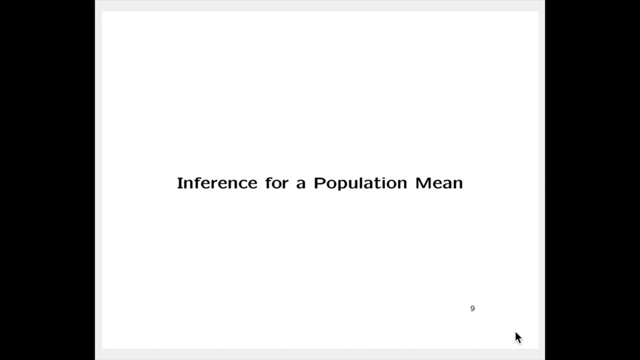 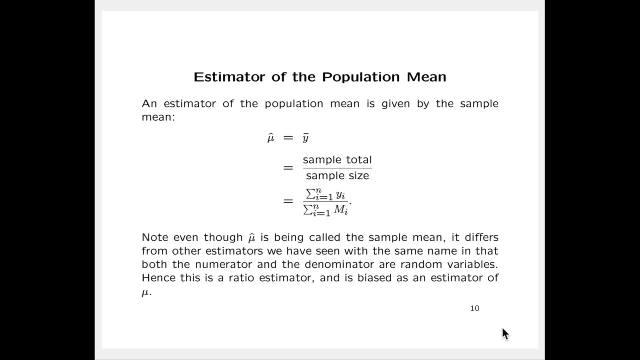 Here we find that 2er plus m bar is just n minus m over n plus n at the end of the cluster. so first we maybe square some stretches right up the middle of the cluster, Then you set up two of these slants for your 그때. The first one is where the sample number falls. The second one is the weight of the riesica discoloration. It closes eachättast auch by sides, and so down over this unity defaults into x the total. total difference between the cluster and the number of members within the sample. 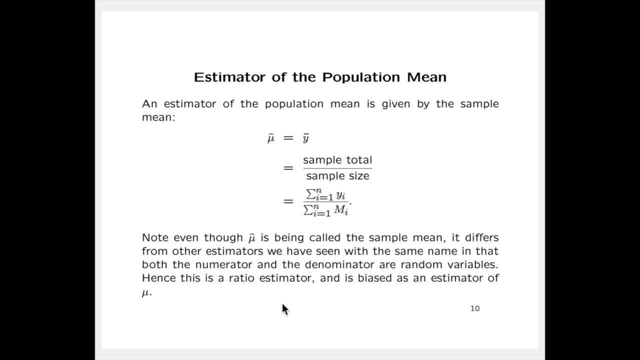 The reason the start and photos are 68% is because the score is the same. We have that use of the cluster size by legendly количеizing, not too surprising. We will denote the estimator of mu by mu hat, and it's equal to y bar. 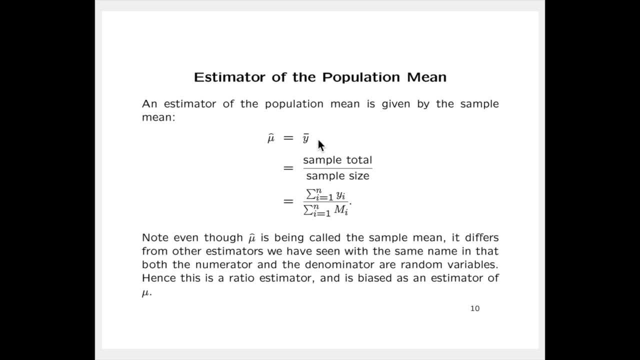 which is the usual notation for the sample mean, when we're using y's to represent the response variable. Remember the y sub i's are actually the total of the response in a given selected cluster. Now, in words, y bar is equal to the sample total. 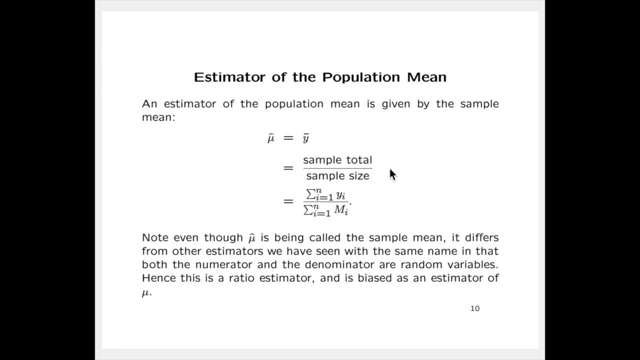 divided by the sample size, and that is typical. That's what the sample mean usually is All right, let's look and see how that works out, or what it looks like mathematically using the notation. So the sample total is the sum of the y sub i's. 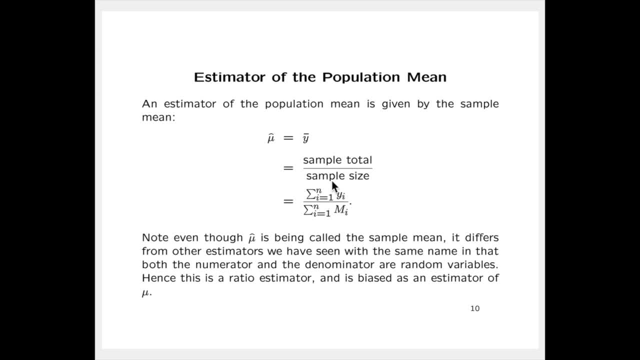 i going from one to little n, So it's the sum of the cluster totals for the cluster selected for the sample. And then we divide that by the sum- i going from one to little n- of the cap m sub i's All right, and again the cap m sub i. 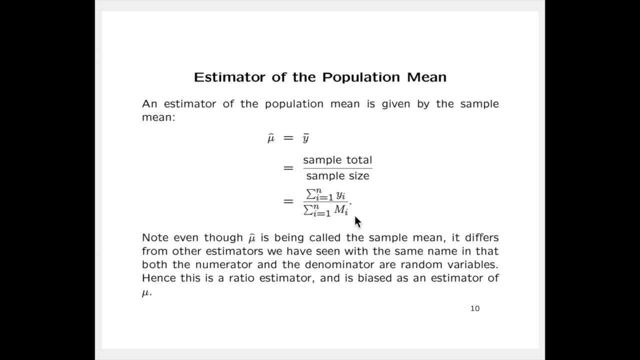 is the size of the ith cluster. So the thing I want to point out here is that even though we're calling mu hat the sample mean it differs from other estimators we've seen with that same name in that both the numerator and the denominator. 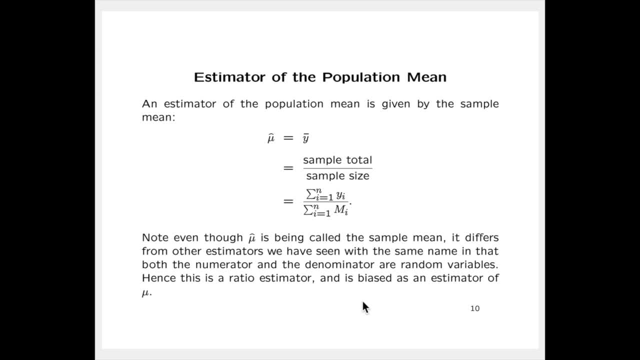 are random variables. Now, that's typically not the case. Typically, we would have the sum of the response divided by, for example, little n- all right- which is typically used to denote the sample size, And, in that framework, the little n. 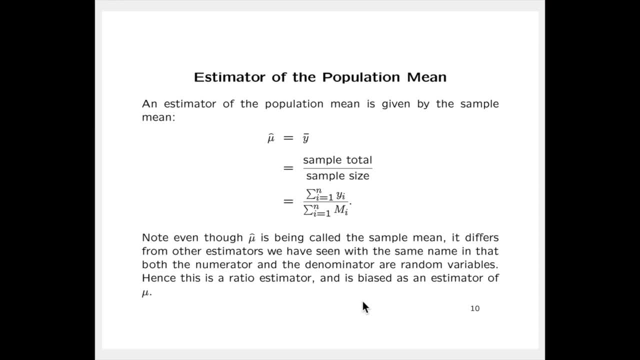 is not random. right, It's not a random variable. The numerator is random, but the denominator is not. But here in this setup, because we're selecting clusters and the denominator of this quantity is the total number of members across the clusters that are selected, 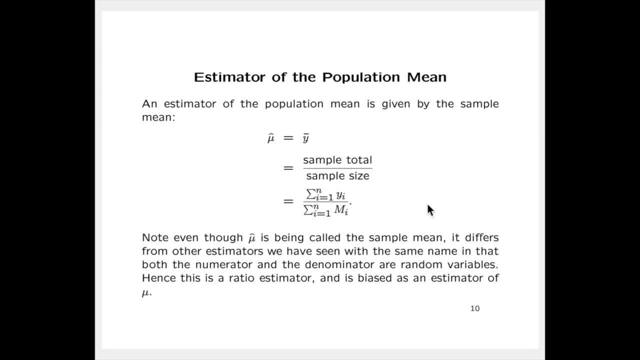 that is also a random variable, okay, And so, because of that, one result of that is that this estimator, mu hat, which is y bar the sample mean, is not an unbiased estimator of mu. It's biased, all right. 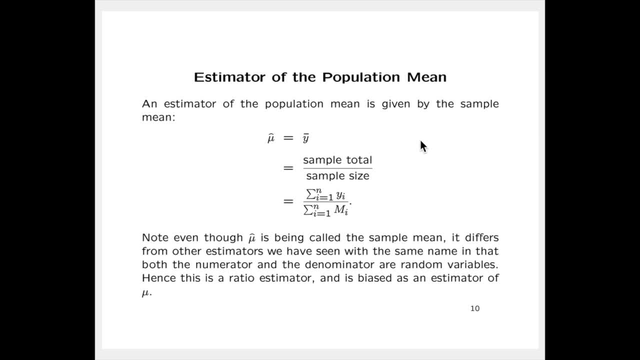 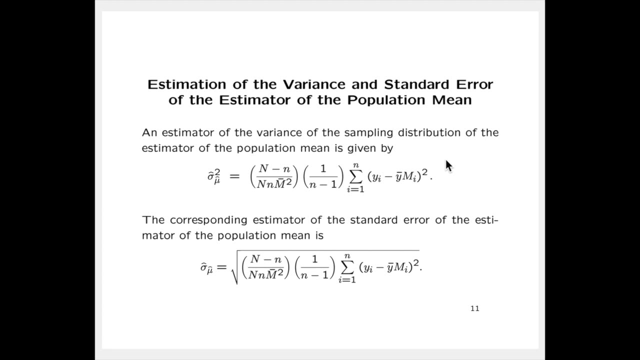 It's a. this is a form of a ratio estimator right, And because the numerator and denominator are random variables, this is not unbiased as an estimator of mu. Now, an estimator of the variance of the sampling distribution of mu hat the estimator of the population mean. 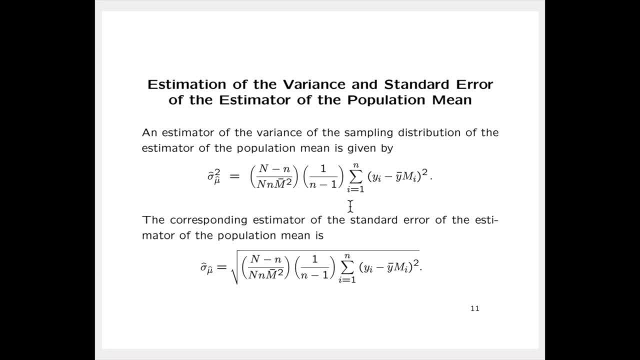 is given here on slide 11,. all right, And so it is this expression. here we'll denote the estimated variance of mu hat by sigma hat squared sub mu hat, as we've done before, And so note that this involves cap N. 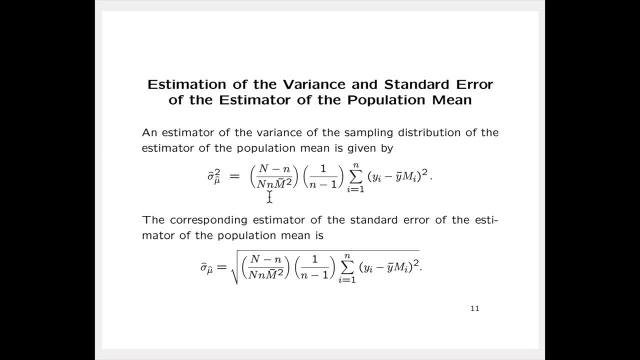 which is the total number of clusters in the population. It involves little n the number of clusters selected for the sample. It involves the square of cap M bar. Remember, cap M bar is the average cluster size in the population. And then it involves this sum. 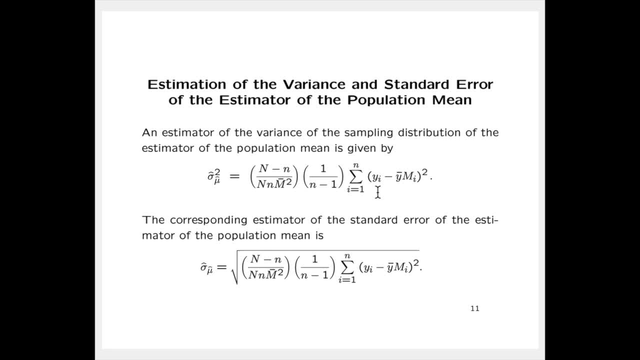 on the right-hand side here the sum of squared deviations between each y sub i and y bar times cap M sub i, And we'll talk about how to efficiently calculate this in just a second Once we have this estimator of the variance of the sampling distribution of mu hat. 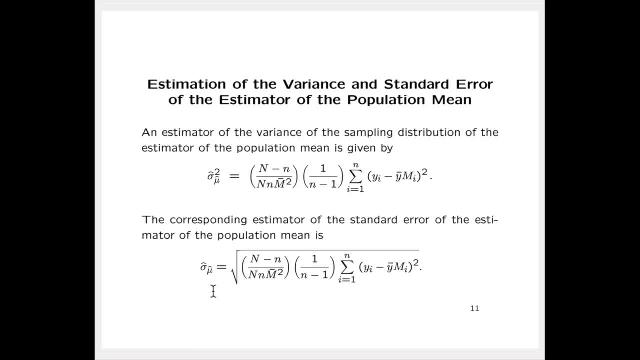 then we take the square root of that to get the estimated standard error of mu hat. Now keep in mind that this estimator of the variance of the sampling distribution of mu hat is not unbiased. Now that expression on the right-hand side of that. 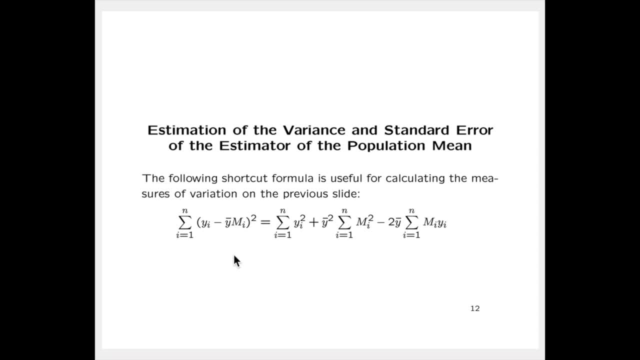 for the variance of the sampling distribution of mu hat. this sum here can be expanded and then calculated using this expansion, so that we don't have to take these differences and square them up. So we calculate the various summary statistics that are listed here and then we use this expansion formula. 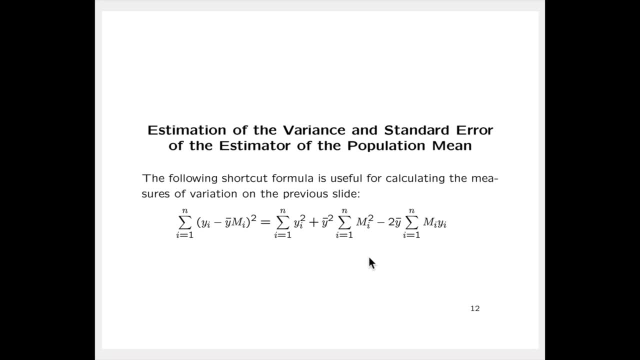 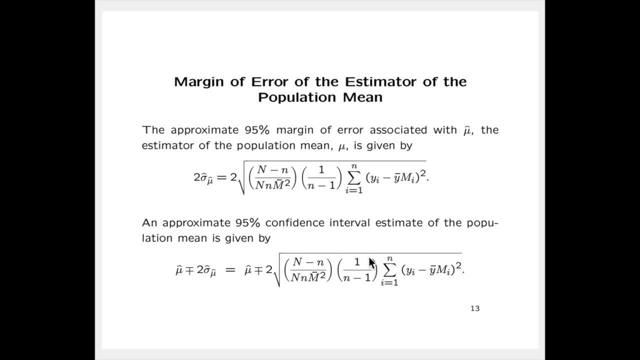 to calculate that sum of squared deviations And that'll allow us to calculate that much, much easier and more efficiently. Once we have the estimated standard error of mu hat, then we can multiply that by two to get our approximate 95% margin of error. 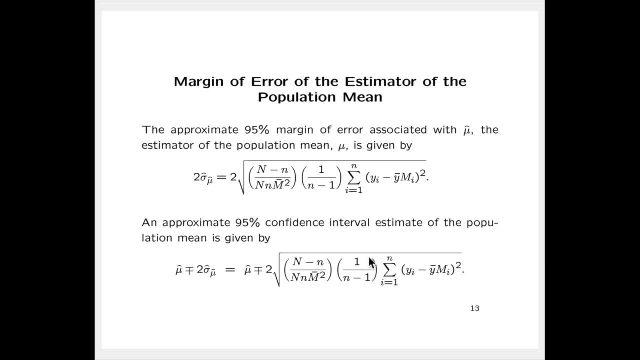 associated with mu hat, And from there we can also construct an approximate 95% confidence interval estimate for mu. And so here on slide 13 is the expression for the approximate 95% margin of error associated with mu hat. And then we have at the bottom of the slide 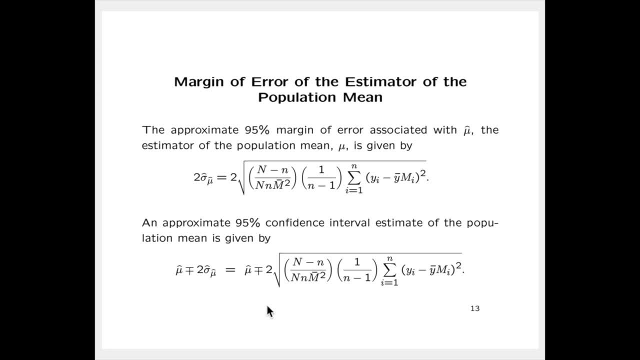 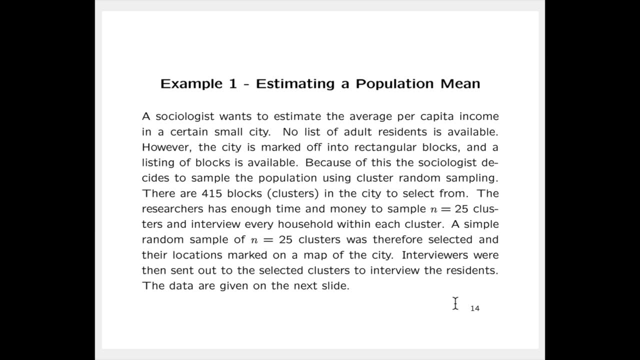 we have the formula for obtaining the endpoints of an approximate 95% confidence interval estimate for mu. All right, so let's look at an example, an application of this. A sociologist wants to estimate the average per capita income in a certain small city. 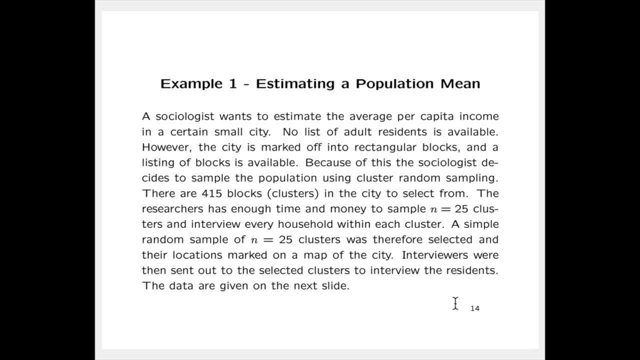 No list of adult residents is available. However, the city is marked off into rectangular blocks and a listing of blocks is available. Because of this, the sociologist decides to sample the population using cluster random sampling. There are 415 blocks or clusters in the city to select from. 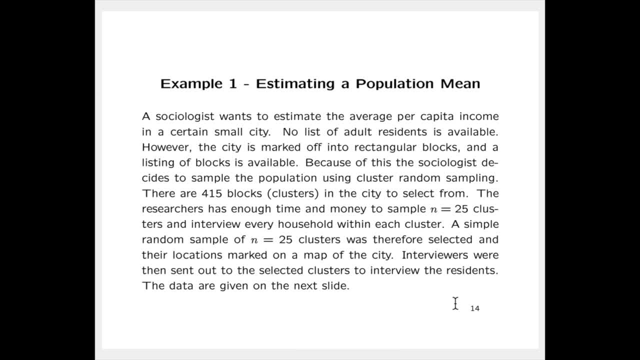 The researchers had enough time and enough money to sample 25 clusters and to interview every household within each cluster. A simple, random sample of 25 clusters was therefore selected and their locations marked on a map of the city. Interviewers were then sent out to. 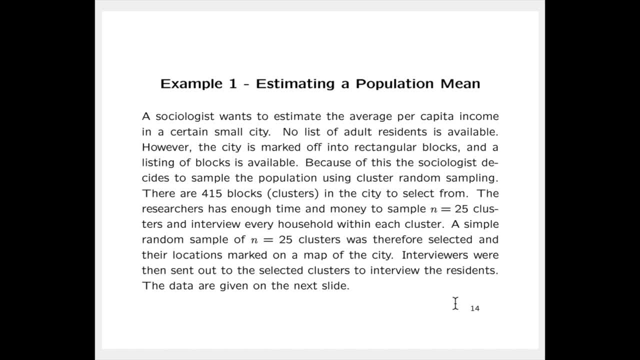 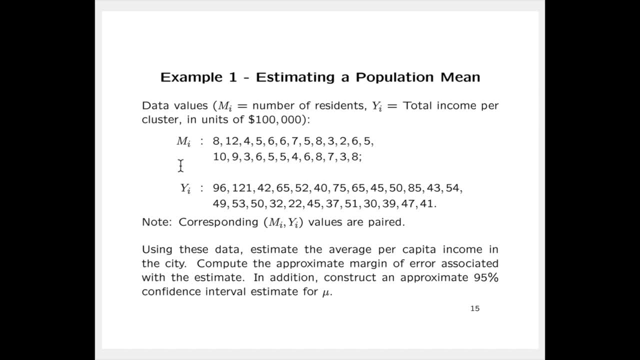 the selected clusters to interview the residents. The data are given on the next slide, And so here we have the data, and the data are paired: Cap M sub I is the number of residents on the selected block And then Y sub I is the total income per cluster. 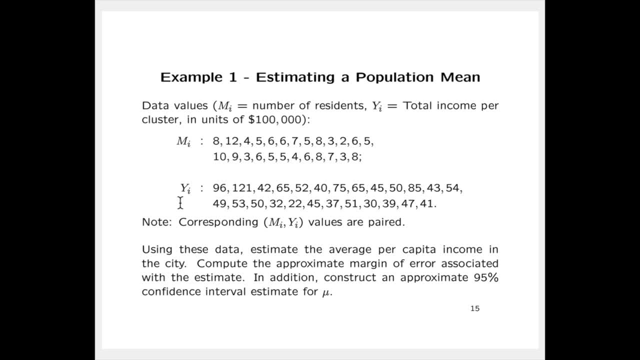 in units of hundreds of thousands of dollars. Okay, so the corresponding M sub I and Y sub I values are paired. So, for example, the eight, the value of eight for M1, and the value of 96 for Y1 are paired. 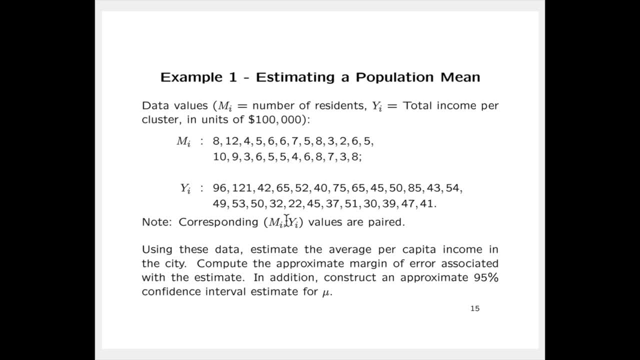 as are the 12 and the 121,, the four and the 42, and so forth. Using these data, estimate the average per capita income in the city. compute the approximate margin of error associated with the estimate. In addition, construct an approximate 95%. 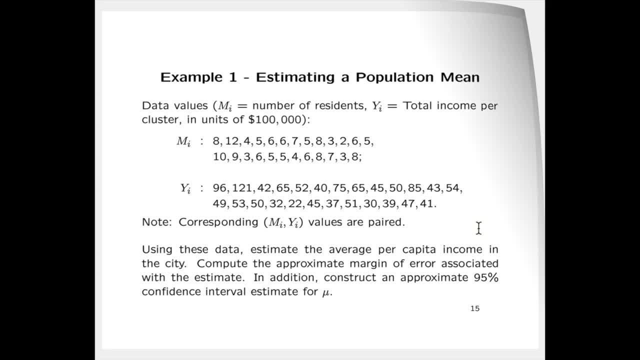 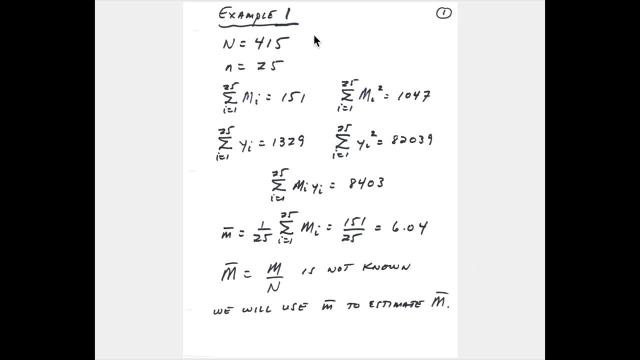 compensative estimate for mu. Okay, so here are the various summary statistics and information available to you. Thank you, And so here's the summary statistics. So again we have. we know that we have 415 blocks in the city. They've selected a sample of 25 blocks. 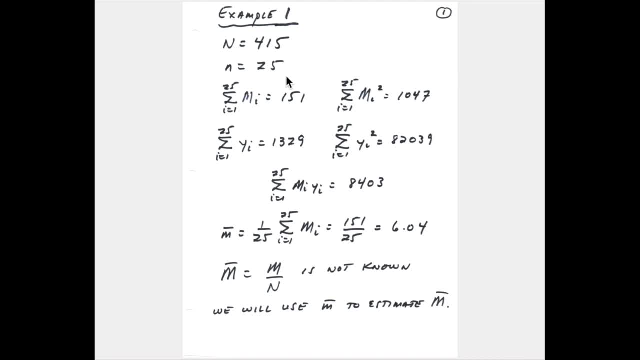 All right, the sum of the M sub I. so this is the number of people. the total number of people selected in the 25 blocks is 151.. The sum of the squared M sub I values is 1,047.. All right, the sum of the Y sub I values is 1,329.. 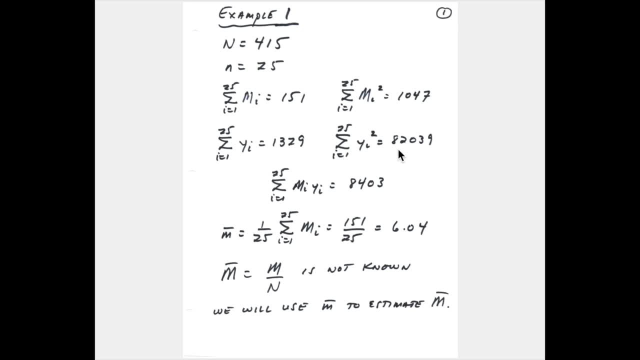 The sum of the squared Y values is 82,039.. And then the sum of the M sub I's times the Y sub I's for the sample is 8,403.. Now little M bar, which is the average cluster size in the sample, is 6.04.. 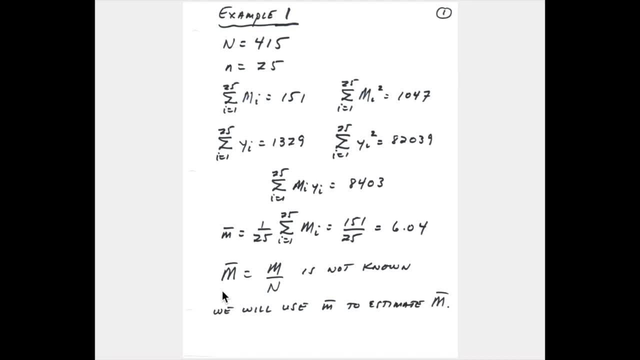 All right, and cap M bar, which is the average cluster size in the population, is not known. and it's not known because we don't know cap M, And so the formula, the formulas that we're using, require cap M bar or an estimate of it. 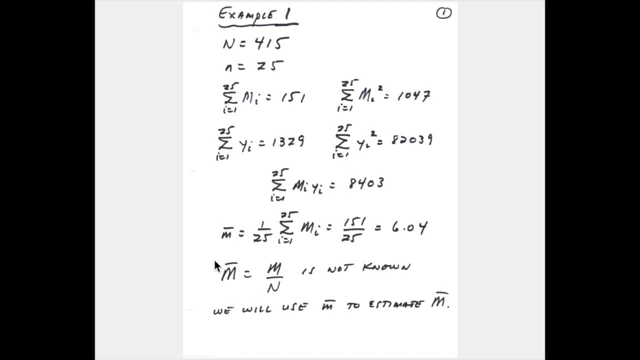 And since we don't have cap M bar, we're going to have to use an estimate of cap M bar, and that estimate is going to be provided by little m bar. So again, cap M bar is the average cluster size in the population. 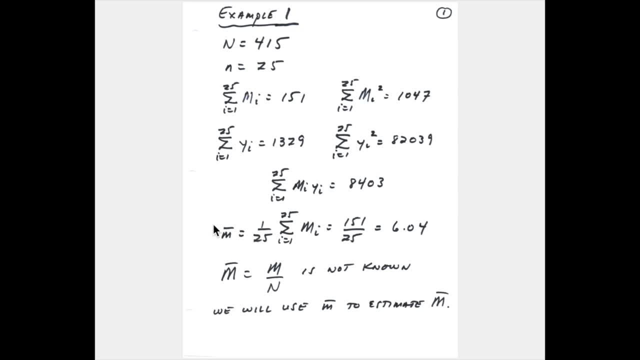 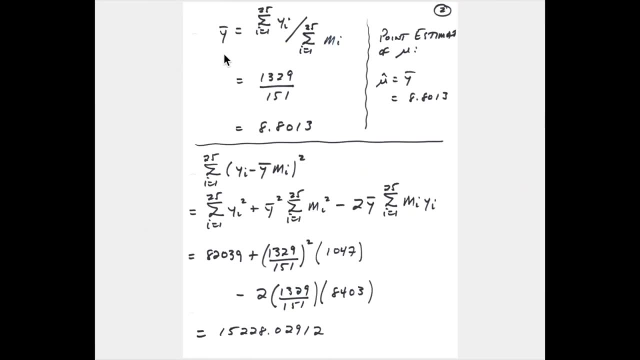 We don't know that, but we do know the average cluster size in the sample, and so we'll use little m bar as an estimate of cap M bar. Okay, Y bar, which is the sample mean, is calculated as the sum of the Y sub I values divided by the sum. 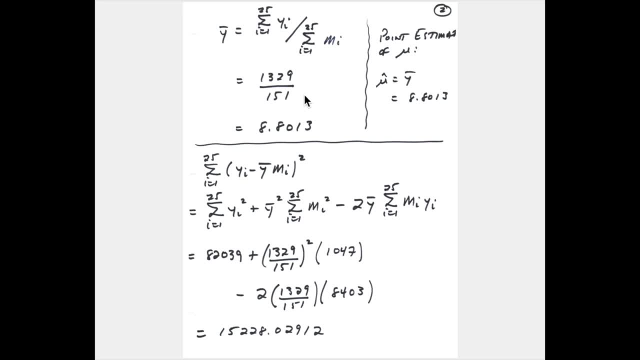 of the cap M sub I values All right, so 1329 over 151, and so we have 8.8013. And so a point estimate of mu mu hat is equal to 8.8013.. So remember that mu is the average per capita income in the 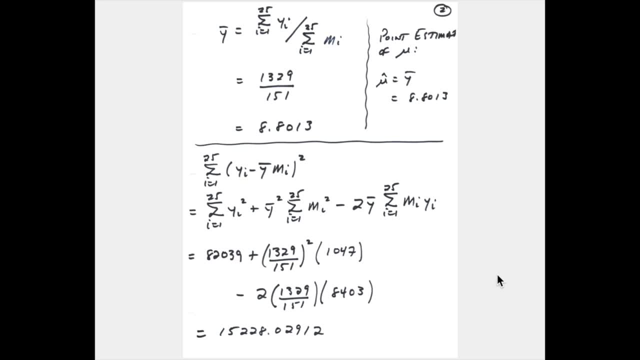 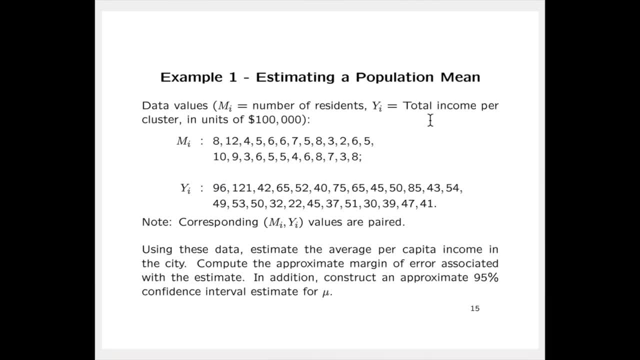 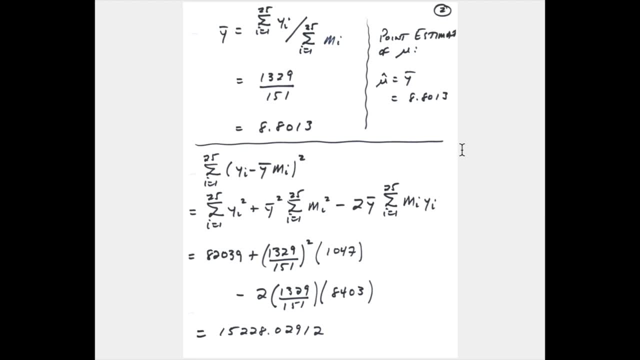 the units of the Y values is income in units of $100,000.. All right, and so what this is saying is that our point estimate for the average per capita income in this particular population is $880,000. essentially All right, so this is a pretty affluent community. 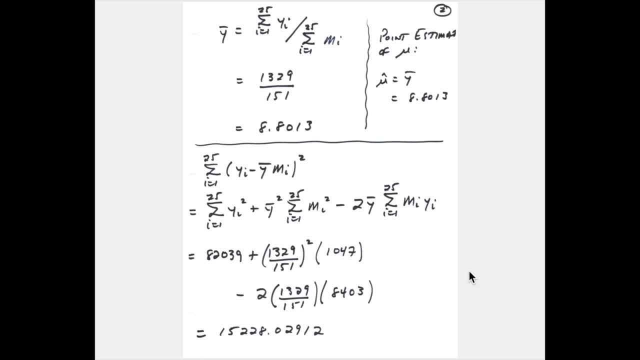 Now to calculate the estimated variance of mu hat, it's standard error and approximate 95% margin of error associated with mu hat, We have to calculate this sum of squared differences between the Y sub I's and these values here, And we're gonna use this expansion formula. 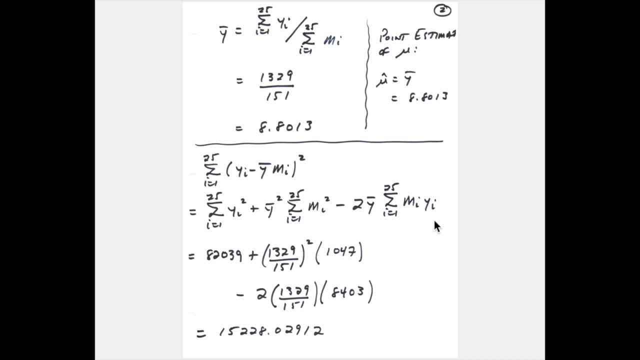 All right, and we have the summary statistics that we need on this page at the top and also on the previous page, And so we plug those in and we get 15,228.02912.. And I'm just carrying out a lot of decimal places here. 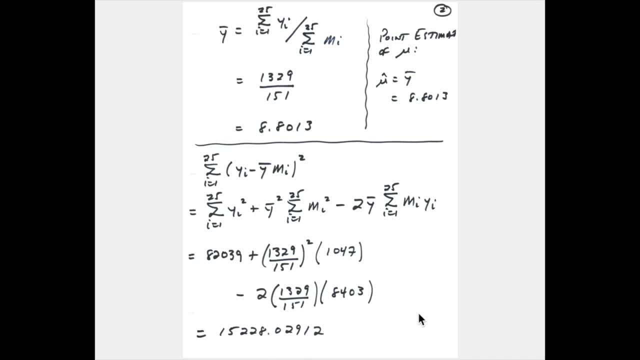 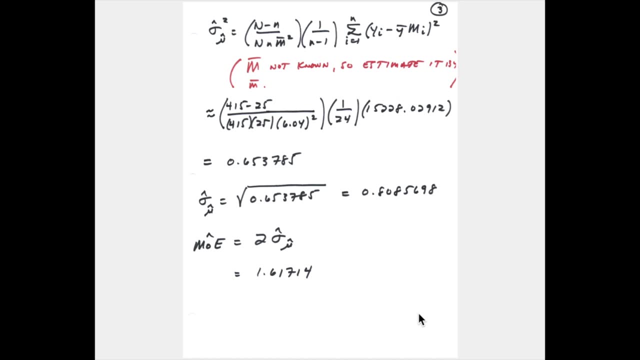 to really reduce any kind of rounding error If I need to. at the end I can always round the final answer. All right, so the estimate of the variance of mu hat okay, given by this formula here. right, we just calculated that sum of squared differences. 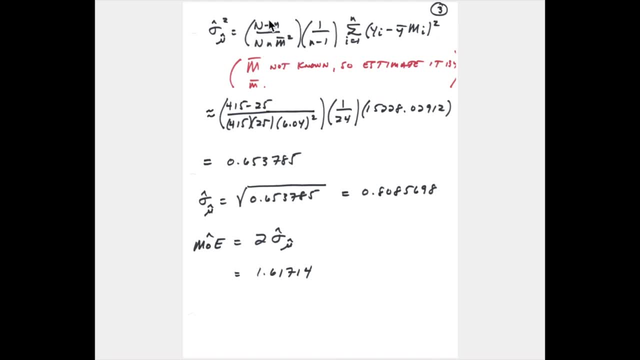 on the previous slide, And we have all the ingredients we need, except cap M bar. All right, we don't know that, And so, remember, we're gonna have to estimate it with little m bar, And so we plug in that 6.04,. 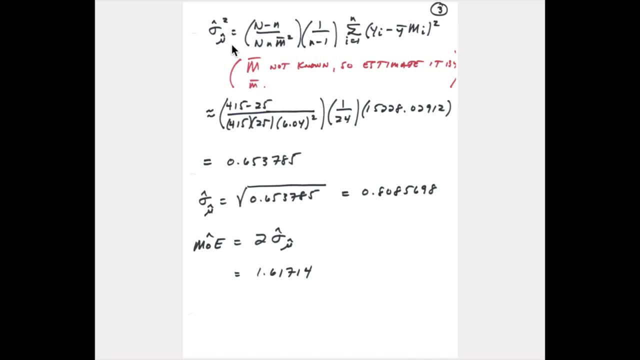 which we calculated a couple of pages ago. All right, and so the estimated variance of mu hat is gonna be approximately equal to- and I've got that approximate there because we're estimating cap M bar by little m bar- So it's approximately 0.653785. 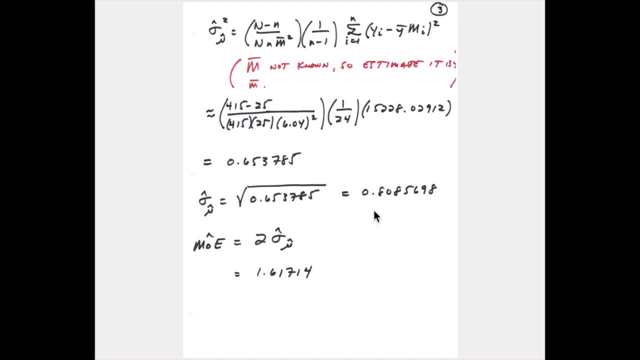 And then we take the square root of that to get the estimated standard error of mu hat, And so that turns out to be 0.8085698.. We then multiply that by two to get our approximate 95% margin of error associated with mu hat.